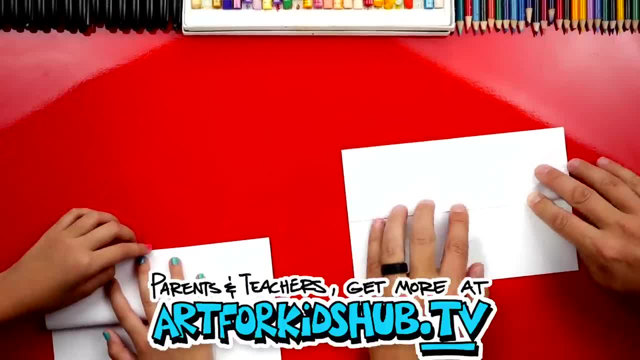 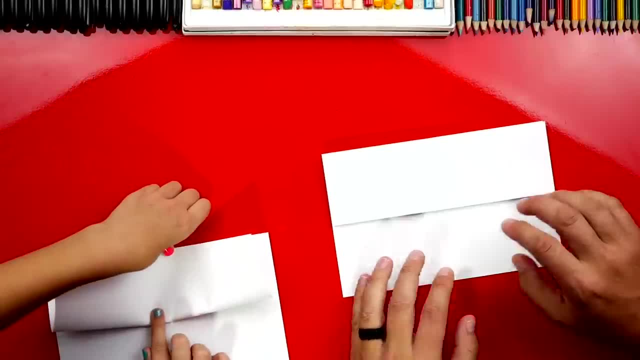 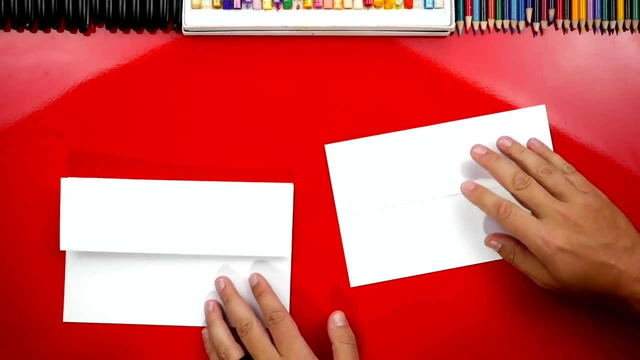 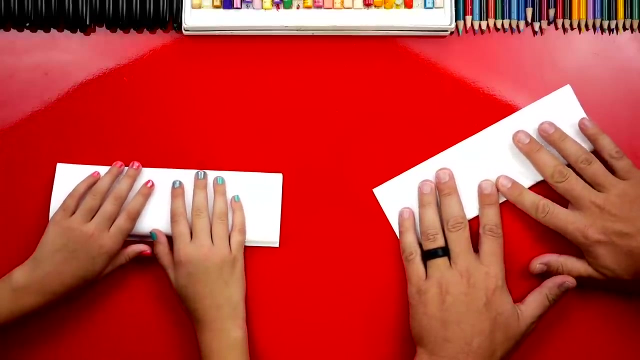 Of our paper. Now, if we ever go too fast or our art friends need more time to finish the step, what can they do? Pause the video. Yeah, you guys can always pause the video or rewind it if you need to see the step over again. There you go, Out to the edge. Alright, now let's flip it over and then we're going to do that step one more time: Fold the bottom edge up to the top and out to the edges. There you go. 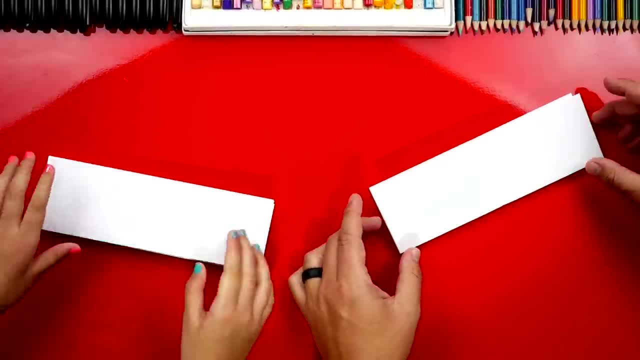 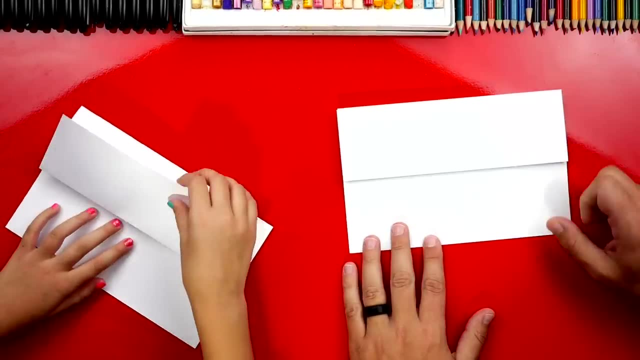 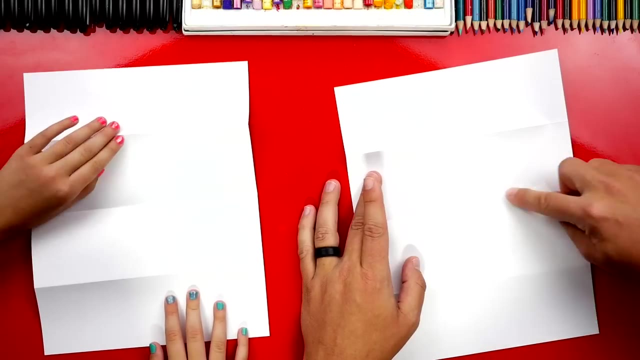 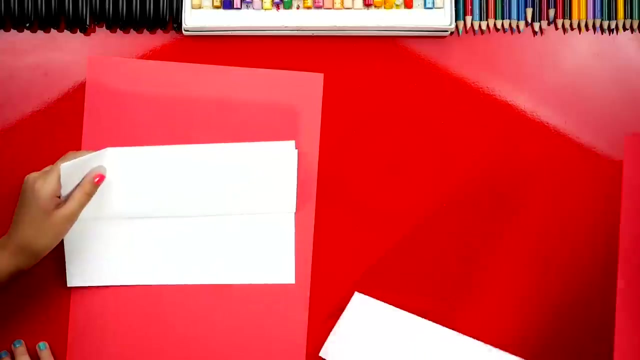 Good, Alright, now that last fold we're just going to use as a guideline. So we're going to open it back up and then you know what we're doing. Flip it back over. Yeah, and if you unfold it all the way, you should have three folds: One: the top, middle and bottom. Let's fold it back up like this. Then we're going to use this scratch piece of paper to put underneath our drawing paper so that when we use our markers it doesn't bleed through and get onto our table. 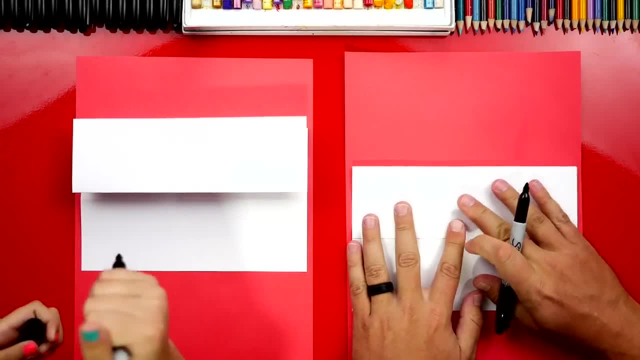 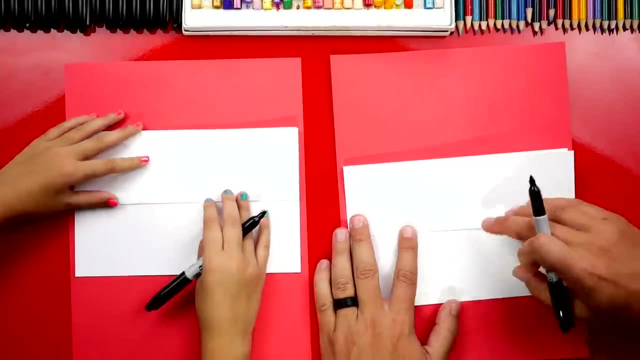 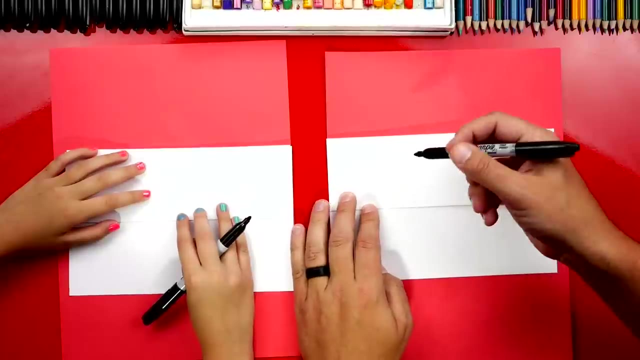 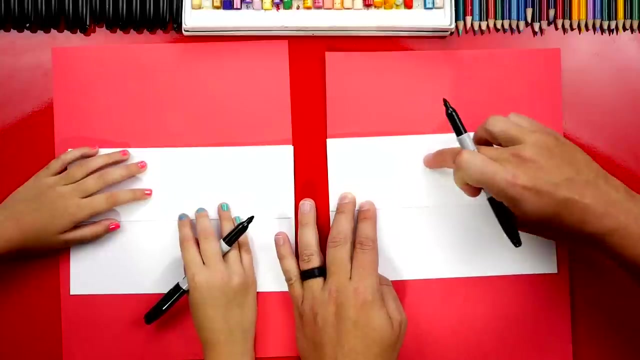 We're going to use our sharpies, but you guys at home can use whatever you feel comfortable: drawing with Pencil or a crayon or even a washable marker. Now we're going to draw a box or a square, and the top of our present is going to be above this fold and the bottom of our present is going to be below. Let's first draw the side of our present. Now, up here, we're going to leave some room at the very top so that we have room for the bow on top of our present. So we'll draw a line that comes down like this: But look at the very bottom. we're going to 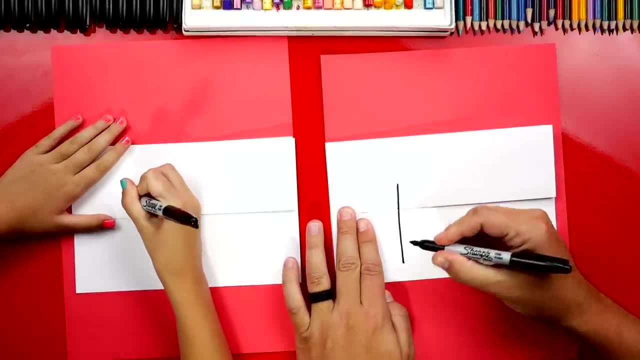 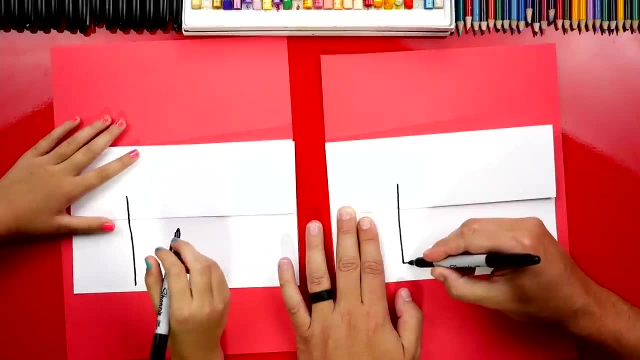 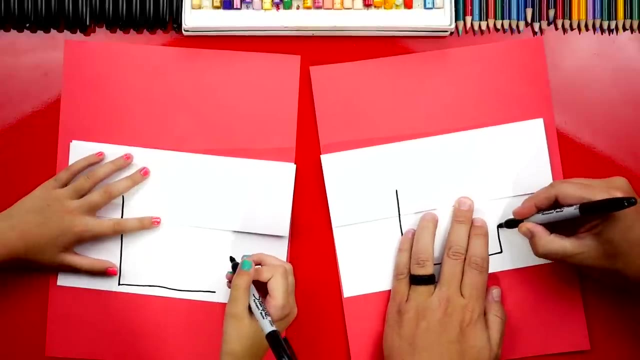 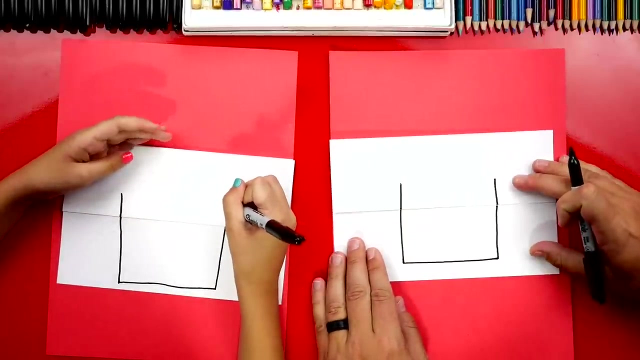 get a little closer to the edge of the paper down here. So leave some space up at the top but get close down at the bottom. Good, Then let's draw the bottom of our present So we'll draw a horizontal line coming across, and then we can draw another line up for the other side of our present and we want it to be the same length as the first line. Yeah, now let's connect the top, Draw another line that goes across. 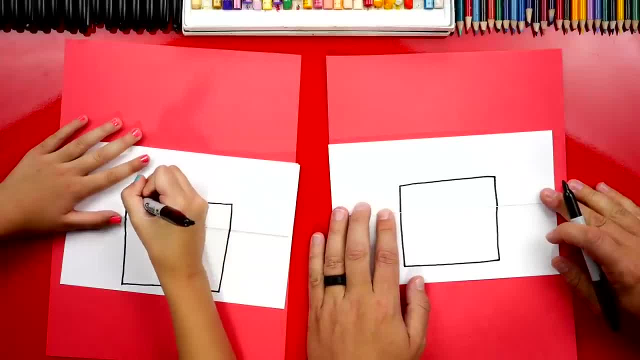 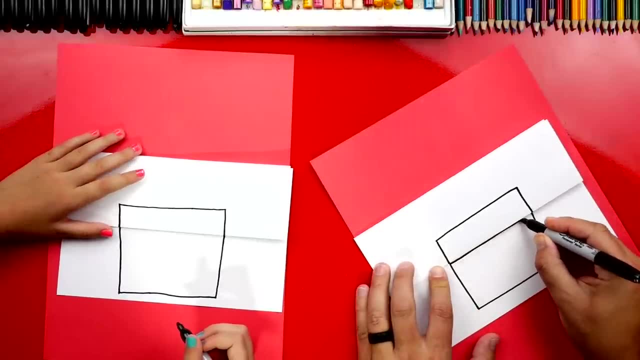 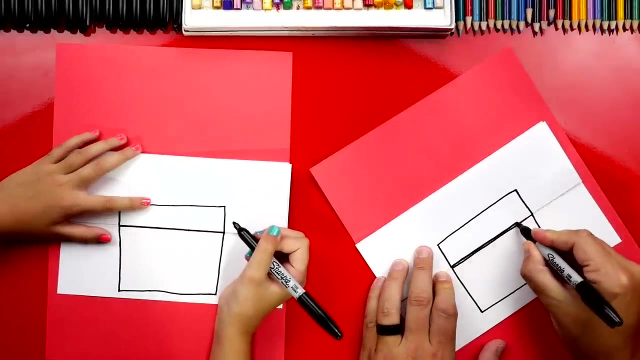 to the other side. All right, now we're going to add a lid to our box. So right here on the fold, let's draw another horizontal line that comes across, and I'm drawing it below the fold, but you can add another line on top of the fold, So you have two lines: one for the top or the lid on our 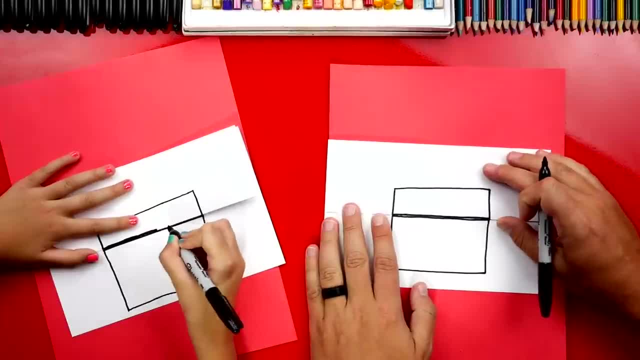 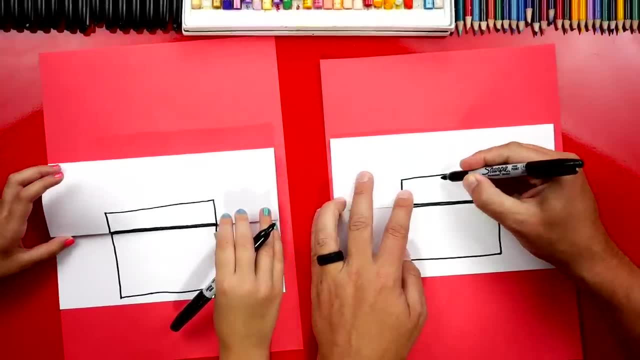 present and one for the bottom of our box. There you go. All right, what's our present? missing A ribbon. Yeah, it just looks like a box. Let's add a ribbon. We're going to draw two lines, vertical lines that come down right next to each other. 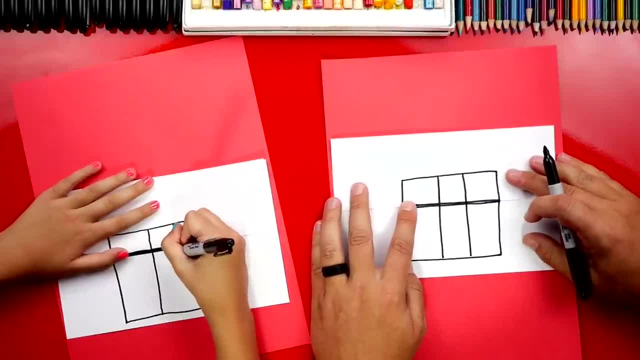 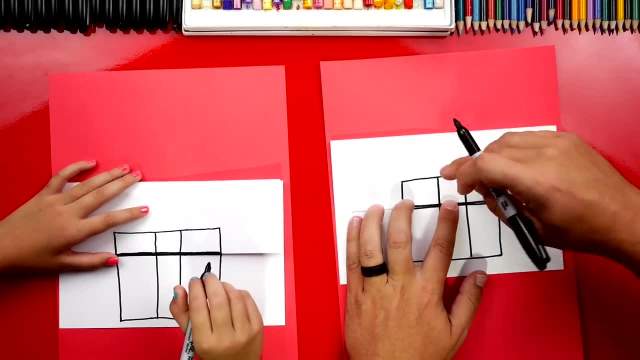 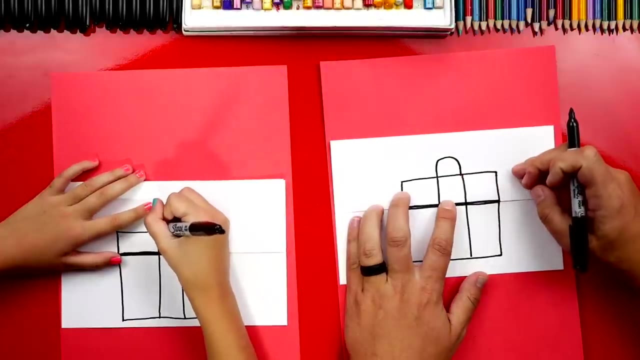 Now these steps are almost exactly like our Christmas present drawing: Oh yeah Yeah, but we're adding it on to our folding surprise. So now let's draw the bow on top, So we'll draw a curve that comes around. This is for the knot in our bow. It kind of looks. 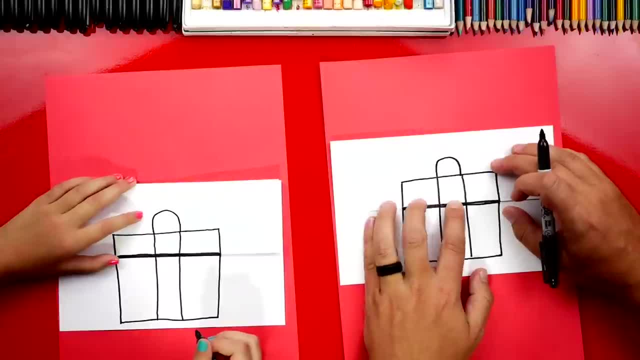 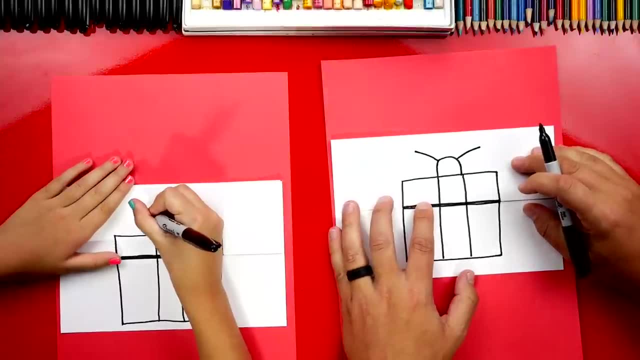 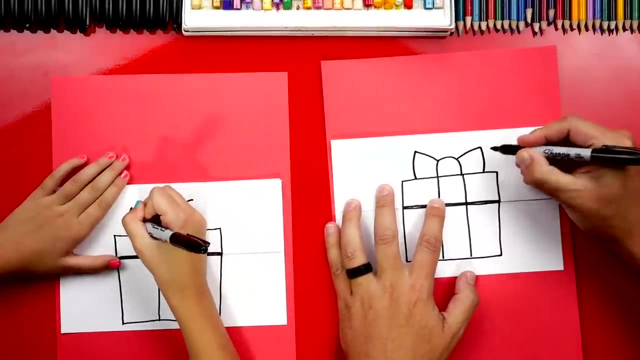 like a marshmallow. It does look like a marshmallow. Now I'm hungry. We can draw a line coming out on each side. Now it looks like an alien or a bug. Let's draw a line that connects down to the box on both sides. 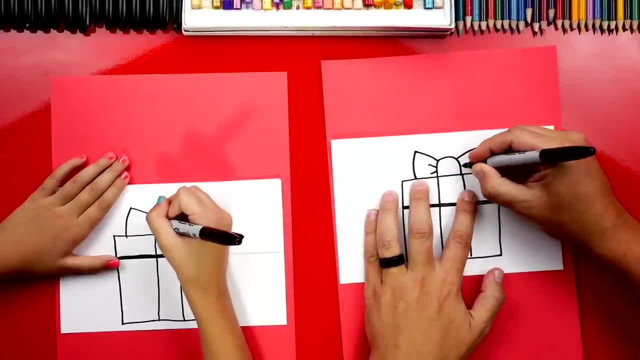 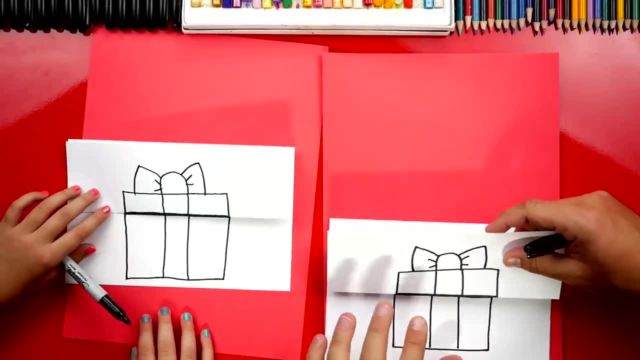 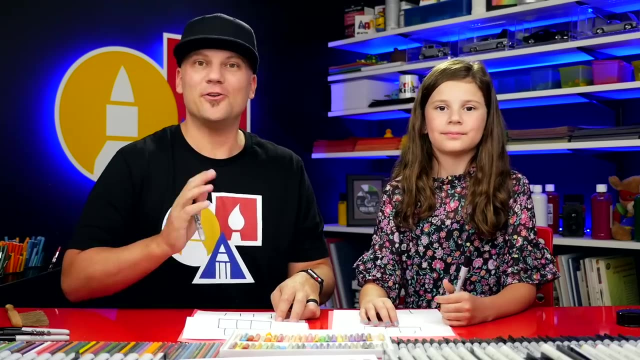 All right, then we can also add two little lines for the wrinkles on the bow. We did it. We finished drawing our birthday present. Let's open it up. and we got all the this extra space in here. What could we put in here? Your favorite toy? Yeah, you. 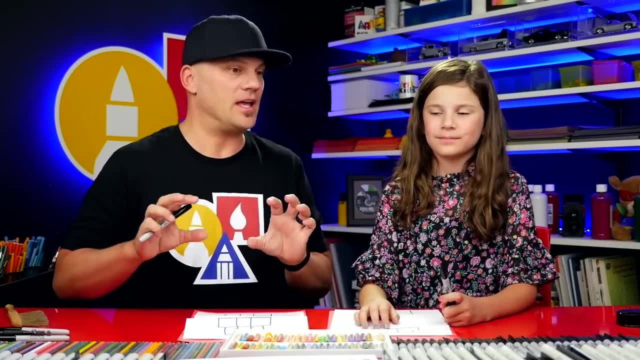 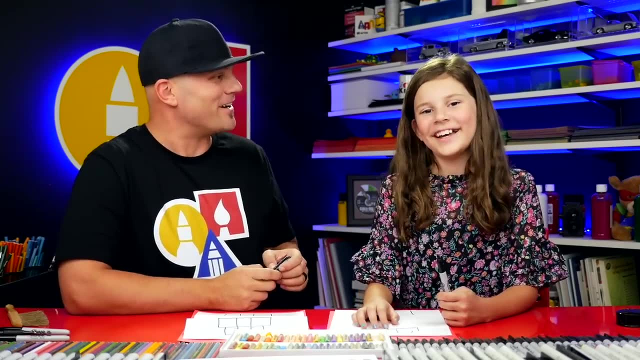 could draw your favorite toy. You could also write the word happy birthday or surprise, or what kind of toy would you put in there? A teddy bear? I like that. Now this part we're gonna fast forward, but at the end, if you want to match the 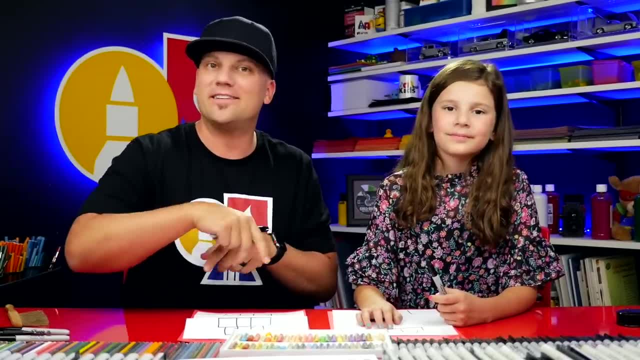 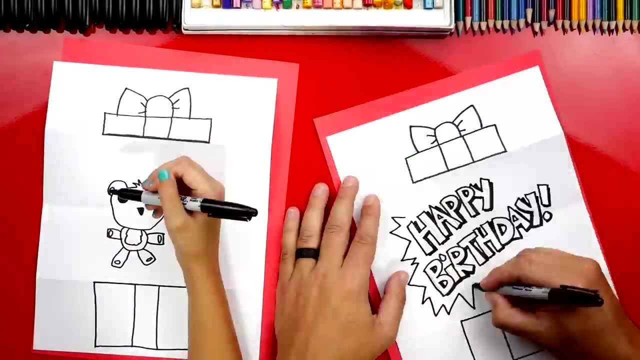 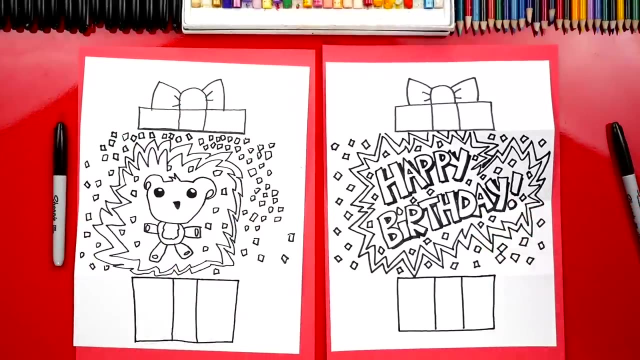 same drawing that we do. you can pause the video or you could use your own creativity and put whatever you want in the folding surprise You ready to fast forward? Yes, All right, Hadley, we did it. We finished drawing our birthday present surprise, but we still need to do one last thing. What is it Color? Yeah, it's gonna look so much.